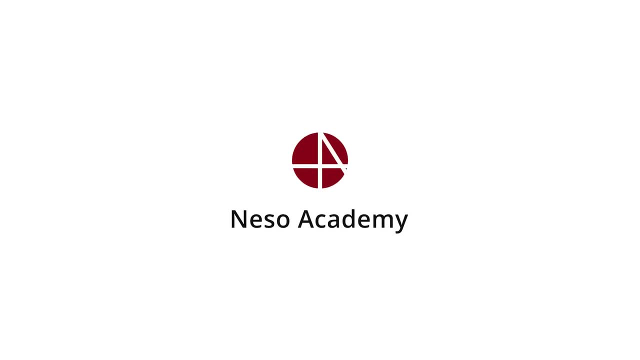 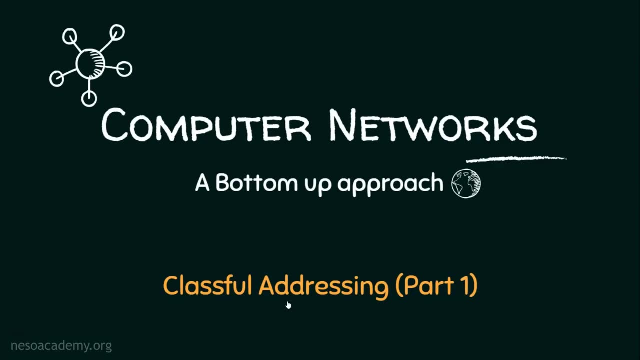 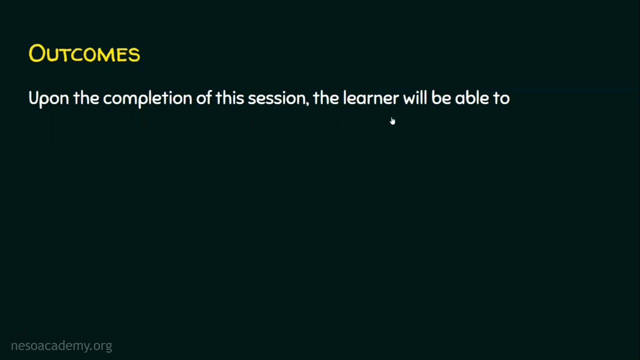 Hello everyone, welcome back. In today's lecture we will see the part 1 of class full addressing. We will start the session with the outcomes. Upon the completion of this session, the learner will be able to outcome number 1,. we will understand various classes of IPv4 address. Outcome number 2,. 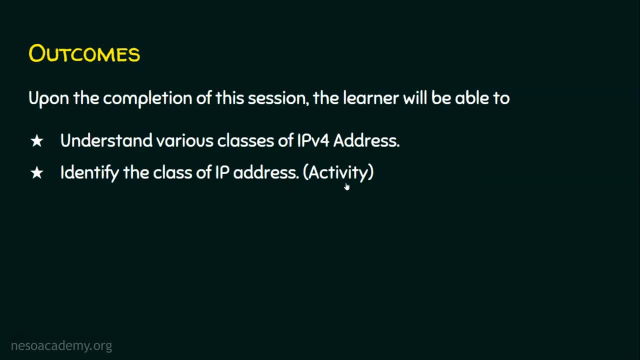 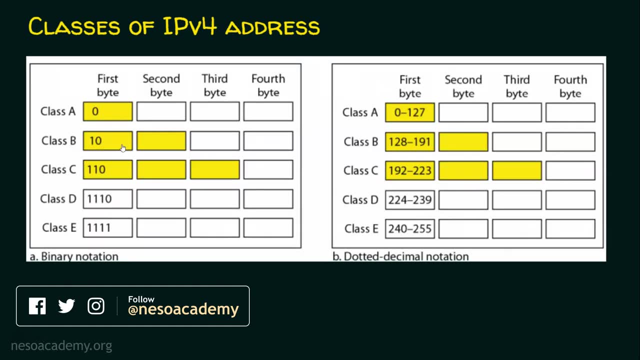 we will identify the class of IP address with the help of an activity. Let's dive into the topic directly. Basically, we have 5 classes of IPv4 addresses: Class A, Class B, Class C, Class D and Class E. We know very well that IPv4 addresses can be represented in two ways. It can be represented: 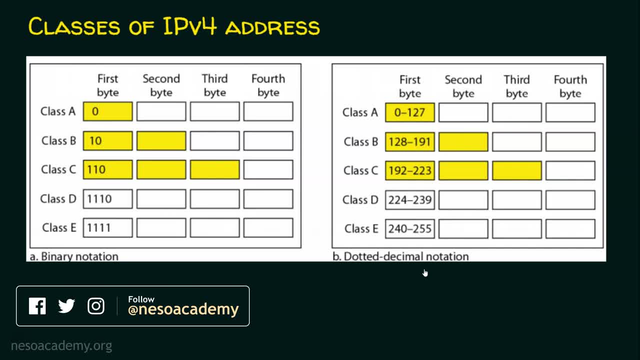 either in binary notation or in dotted decimal notation. We know IPv4 addresses are 32 bits long. These 32 bits are organized into 4 octets, or 4 bytes, and each byte will be 8 bits long. So we have 4 bytes in an IPv4 address. These 4 bytes can also be called as 4 octets, because every 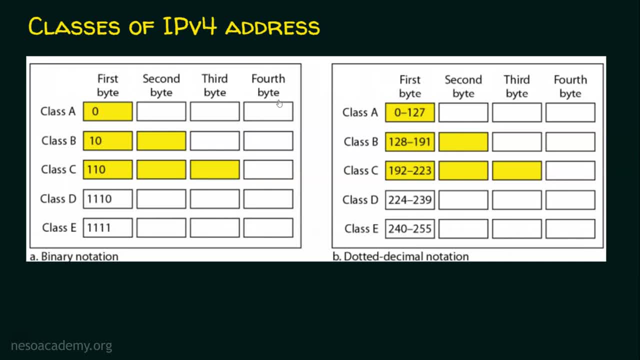 octet is going to contain 8 bits, So 8 plus 8 plus 8 plus 8 is equal to 32 bits, and that's why IPv4 addresses are of 32 bits long And class A means out of these 32 bits. 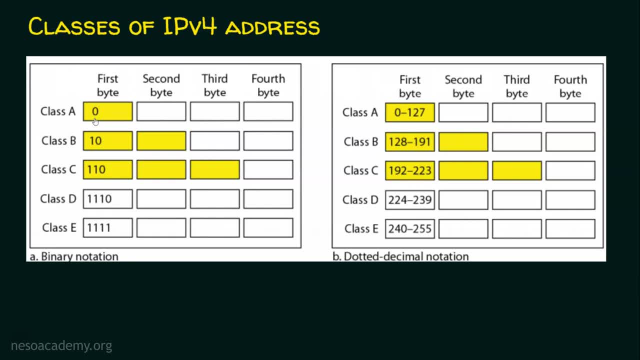 and the first byte. that is the first octet's first bit, the most significant bit. if it is 0, then it is class A. If the first 2 bits in the first byte are 1,, 0, that is the starting of. 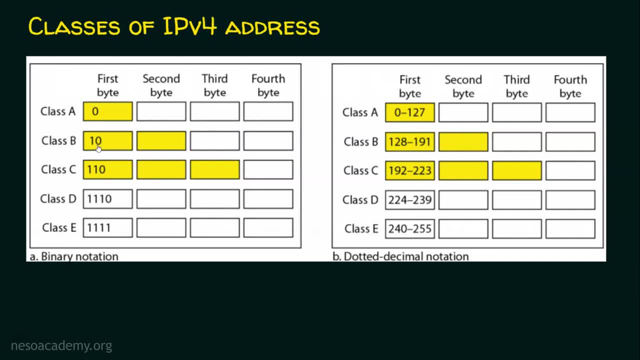 the IPv4 address in binary. if they are 1, 0,, then it do belong to class B. If the first 3 bits are 1, 1, 0,, then it do belong to class C. If it is triple 1, 0,, that is, if the IPv4 address starts. 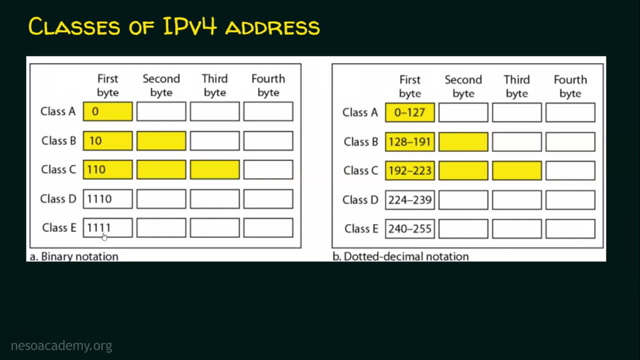 with triple 1, 0,, then it is class D. The first 4 bits of the first byte or the first octet of an IPv4 address are 4 ones. then it is class E. So if it is represented in binary, we need to see: 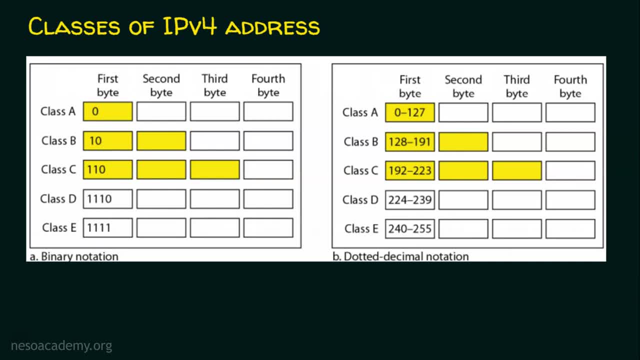 what are the bit values, whether the IP address is belonging to class A, B, C, D or E. In case, if it is given in a dotted decimal notation, say if the first byte or the first octet is between 0 and 127,, it is belonging. 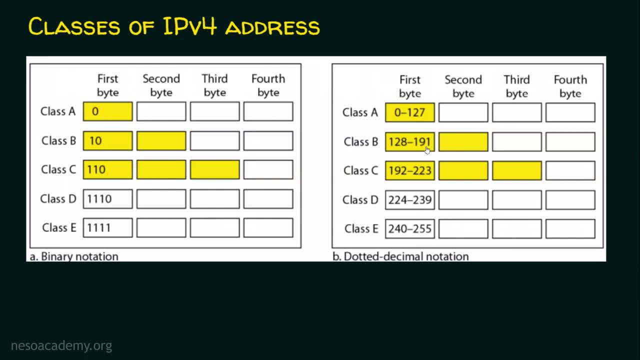 In case: if it is between 128 and 191, it belongs to class B. If it is 192 to 223, it is class C. If it is between 224 and 239, it is class D. And if the first byte or the first octet is between: 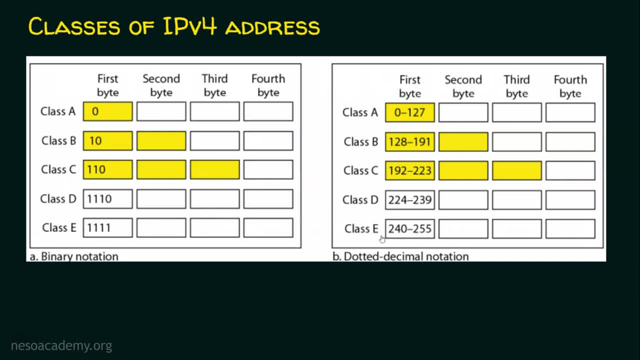 240 and 255, then it is class E. How these values can be generated In an IPv4 address. in a dotted decimal, every octet will be between 0 and 255.. Let's see the various classes of IPv4 address in a detailed. 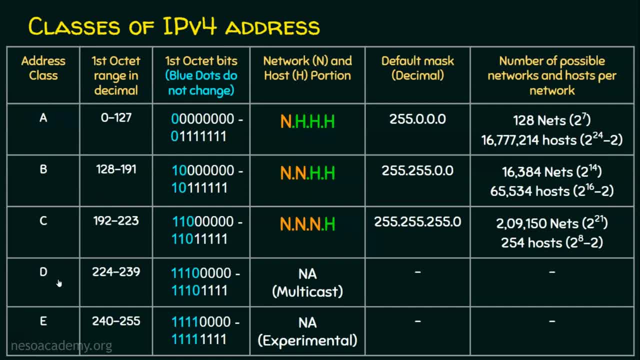 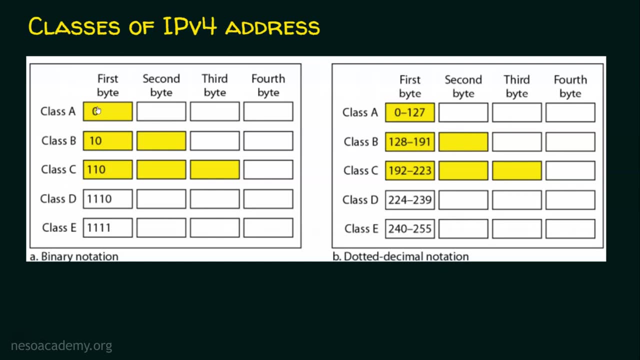 manner. Say, we know we have 5 classes of IPv4 addresses and we have seen in the previous slide that what is the range of each class? We are going to see things elaborately now. We have seen in the previous slide that the class here is first. octet's first bit is fixed, that is, it is 0. So when we 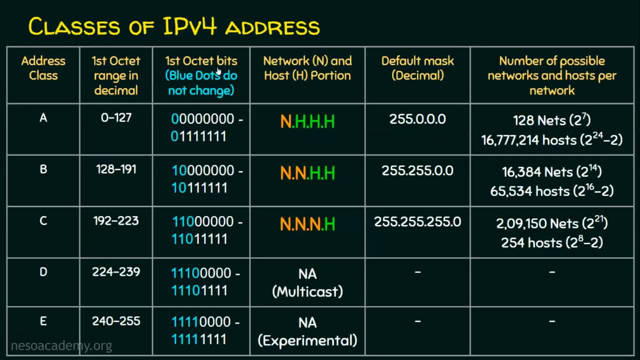 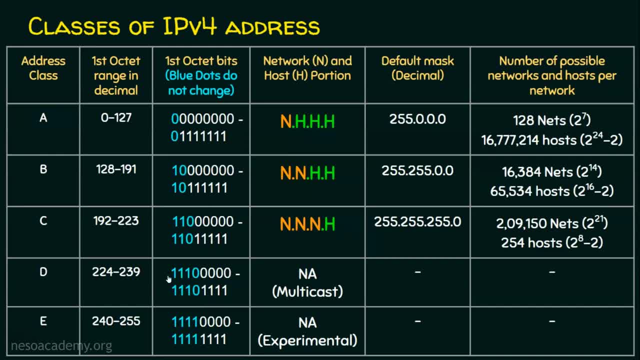 180 and 239 as the ending of IP address in Class D. Let's now move on to Class E. In Class E, we know the starting of the IP address will be all four ones. When all four ones are fixed, we have only. 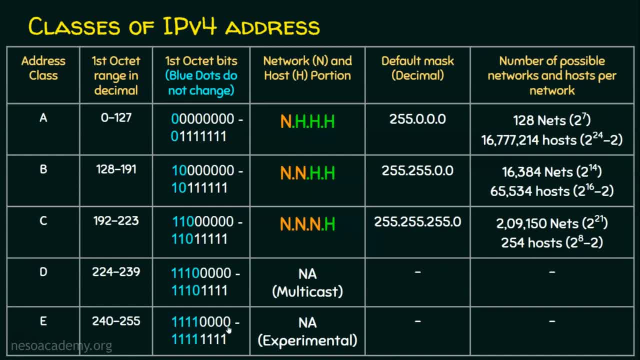 four bits remaining, And these four bits, the starting will be all zeros and the ending will be all ones. And when it is all zero in the last four places of the first octet, then the decimal equivalent will be 240, and the final value will: 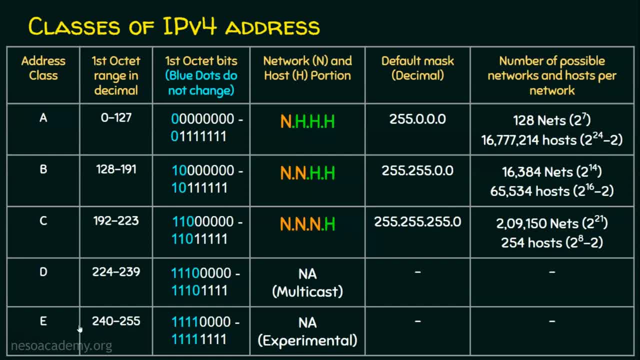 be 2.. So it is real, No 255.. So the starting of class E is 240 and the ending of class E is 255.. And just recall what is the starting value: in an octet, It's 0, right In decimal, it is 0.. And what is the final? 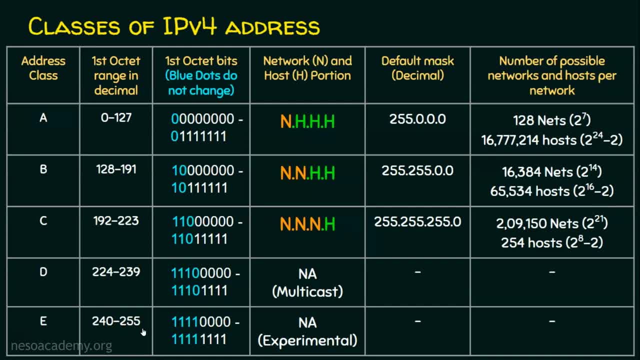 value in an octet It is obviously 255.. Between 0 and 255 in the first octet we have five classes. These- class A, B, C, are for general purpose and class D is for multicasting purpose, and class E. 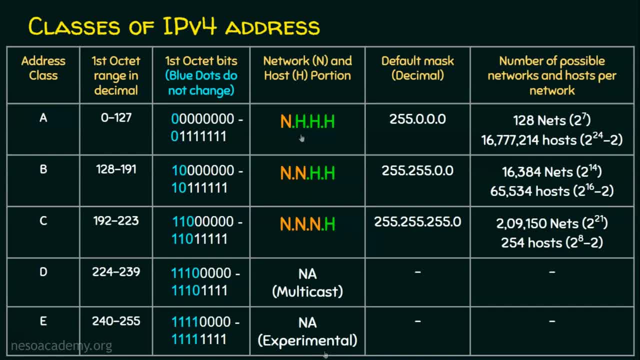 is reserved for experimental and research purpose. I'm not going into the details of these things in this lecture. Anyway, we are going to deal about this elaborately in the next lecture. This lecture is intended to know how many classes and how each class is identified. Let's now move on to the 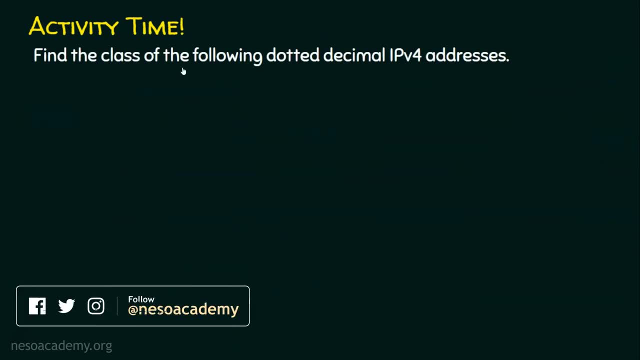 activity. The activity is find the class of the following dotted decimal IPv4 addresses: So we are given with some IPv4 addresses and we are required to identify or find the class of the the IPv4 address. IPv4 addresses can be given either in the dotted decimal format: 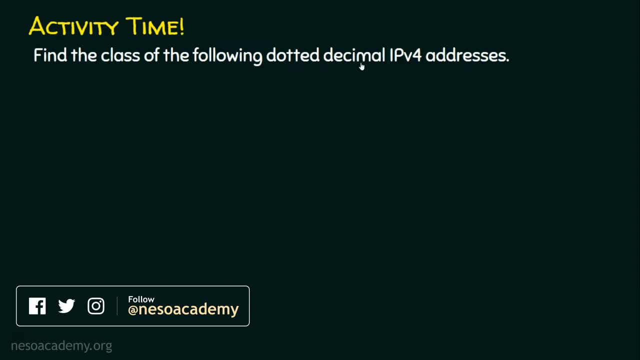 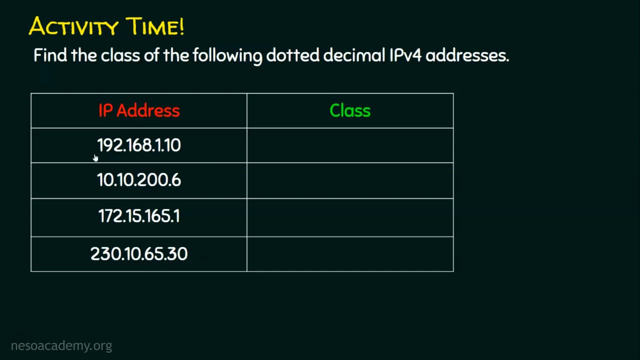 or in the binary format. In this activity, the IPv4 address is given in the dotted decimal format, So these are the IP addresses. given How to identify the class of the IP address, We are required to focus on the first octet. 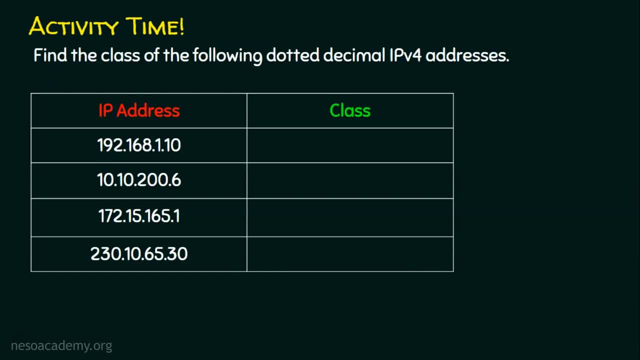 If the first octet is between 0 and 127, it is class A. If it is between 128 and 191, it is class B. If the first octet is between 192 and 223, it is class C. 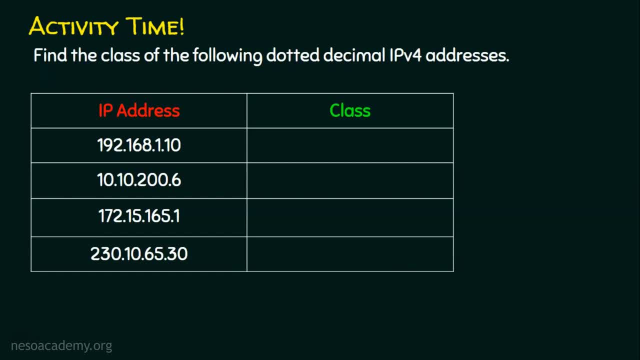 Between 224 and 239, it is class D And between 240 and 255, it is class E. The first octet in this IP address is 192.. So this is between 192 and 223.. So obviously it is class C. 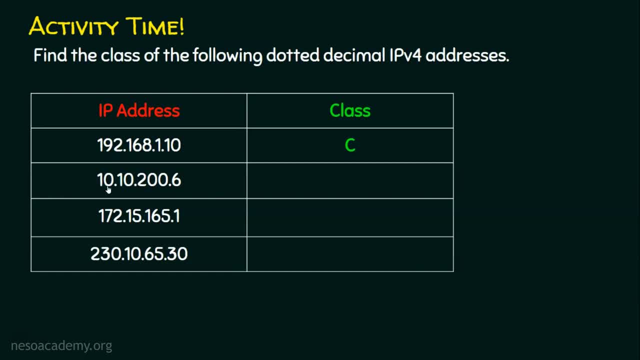 Let's move on to the next value. This is starting with 10.. If the first octet is between 0 and 127, it is class A And coming to the third one, And this octet is between 128 and 191.. 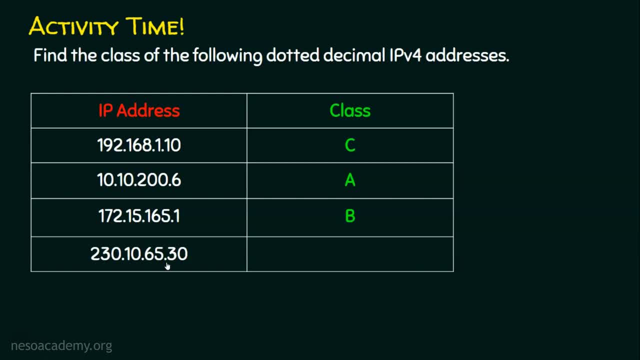 So obviously it is class B And the class for the last IP address is class D. This is a multicast address. Why, If it is between 224 and 239, obviously it is class D, which is mainly reserved for multicast purpose. 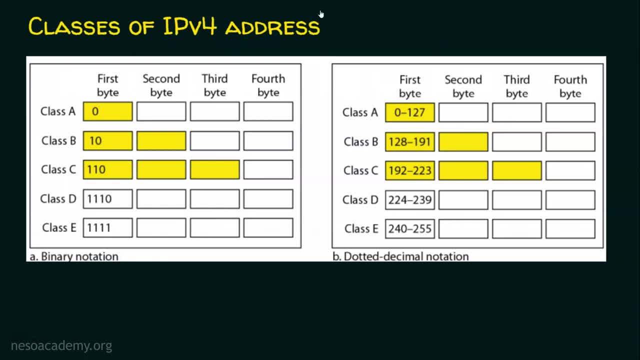 If you want to solve these questions, so you should be very proficient with this table. Just refer the first octet values and identify the class. The question may be given either in the dotted decimal notation or in the binary notation. Now let's see the homework question. 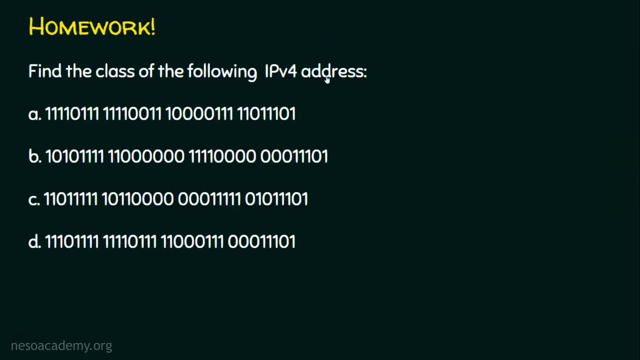 The question is find the class of the following IPv4 addresses And we are given with four IPv4 addresses, But this time the IPv4 addresses are given in the binary notation. Four questions are given. Just observe the bits in the first octet. 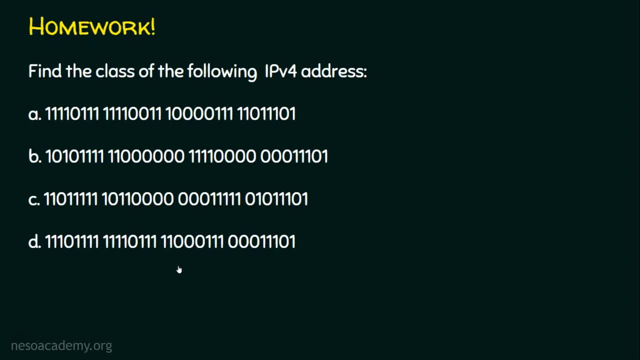 and find the class of this IPv4 addresses. Pause this video for a while, Take the help of this slide and try solving this problem, And post your answers in the comment section. I hope now you understood the various classes of IPv4 address. 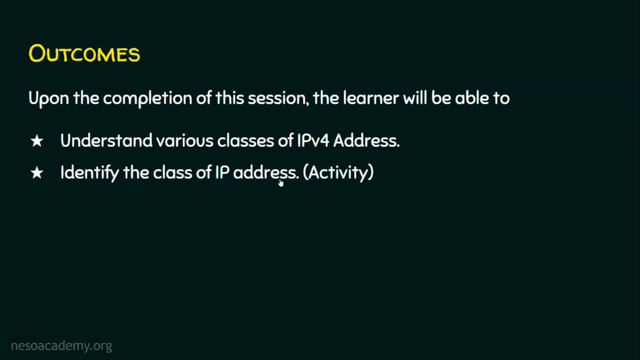 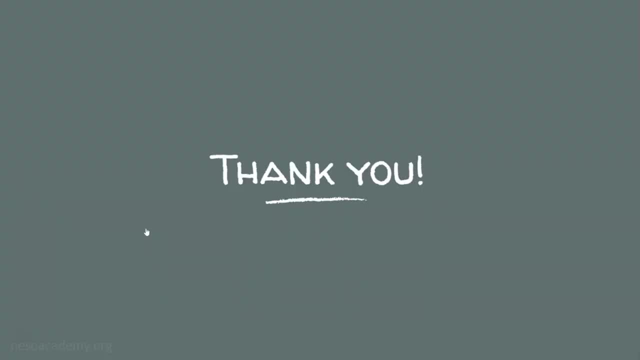 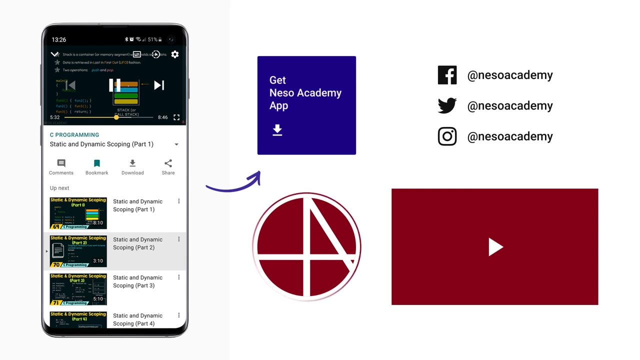 And we will be able to identify the class of IP address if it is given either in the binary form or in the dotted decimal form. I hope you guys enjoyed the lecture and thank you for watching. Bye.